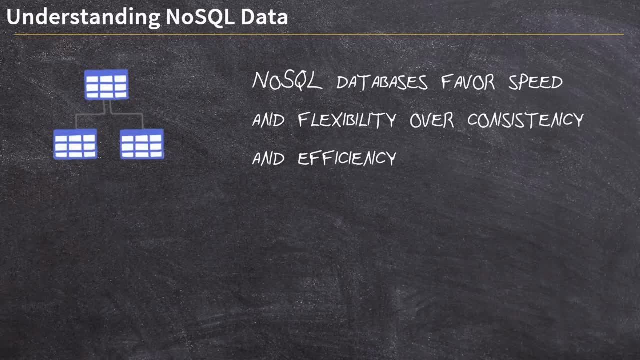 over consistency and efficiency. So consistency and efficiency are two things that I would generally consider to be features of a relational data model. When we talk about NoSQL, we're really talking about speed and flexibility. You're going to hear the word ad hoc a lot, And there's a lot. 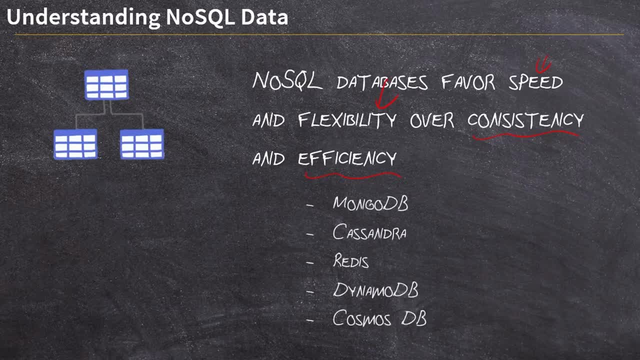 of popular NoSQL databases that are around and available now. You may have heard of some of them. MongoDB, or Cassandra Redis, is a very popular in-memory caching system as well as a key-value pair database, a NoSQL database. DynamoDB is Amazon's. 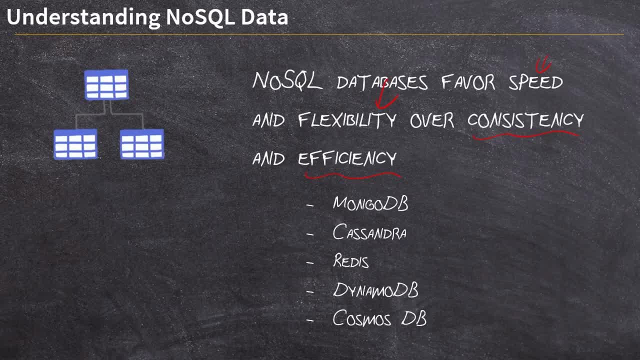 AWS cloud-based NoSQL database service And, in relation to that, CosmosDB is the one from Azure, their cloud-based NoSQL model that's served up on the Azure platform. So these are just some of the different databases. There's a lot of different NoSQL databases that you might run into. 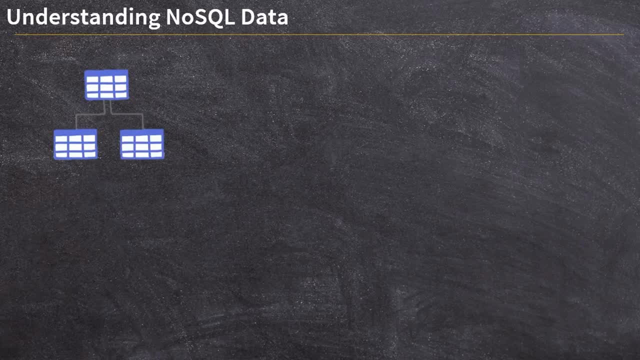 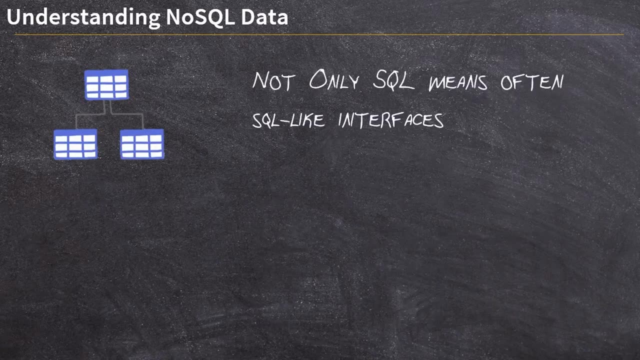 And what makes NoSQL important again is its speed and its flexibility. So if you're looking at a NoSQL database, it's ability to really deal with a lot of different stuff. Now, NoSQL was a phrase that was originally developed to mean NoSQL at all, But really today most people will indicate 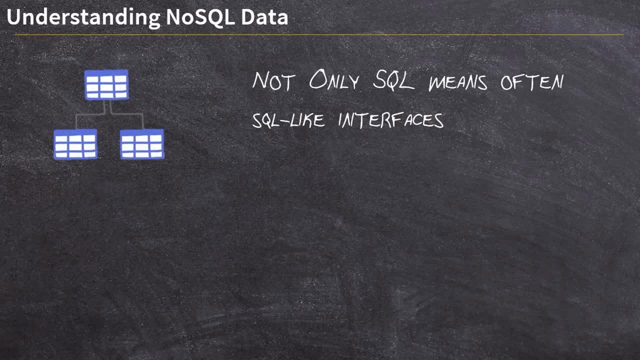 that it means not only SQL. This is really the terminology that's been adopted And that's because usually you're not going to have an SQL interface to NoSQL databases, but you still can. People are very familiar and comfortable with SQL, So a lot of NoSQL databases. 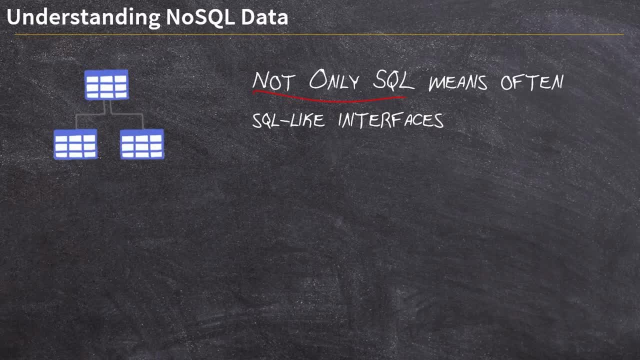 while they don't store in a relational model, will still use the relational SQL language or some variation of it to allow you to interface with that database and put data in or query data out. So you still run into some SQL. Not only SQL is what the NoSQL typically stands for. 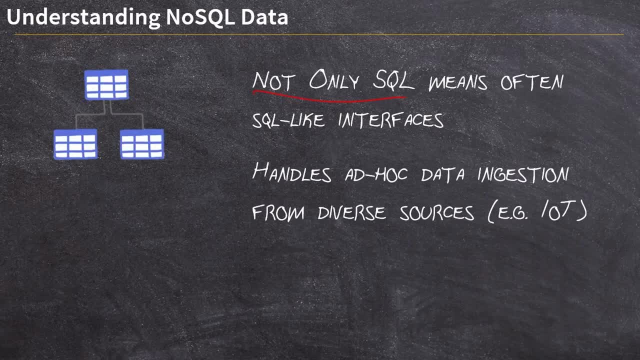 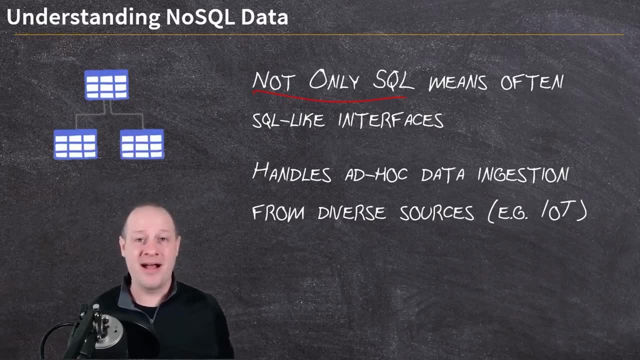 And NoSQL databases like to handle ad hoc data ingestion from a lot of diverse sources. Think about IoT. right, We have all these different devices that might be scattered all over a warehouse. They might be scattered all over the country or even all over the world, And they're 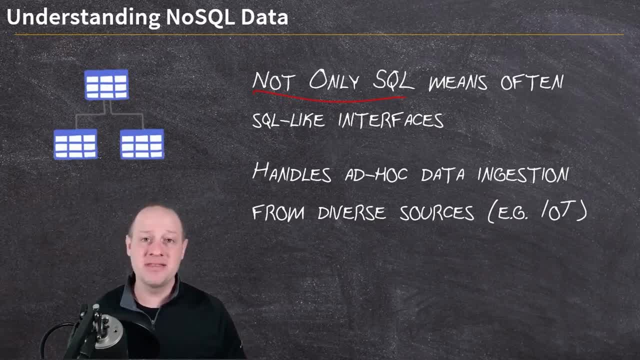 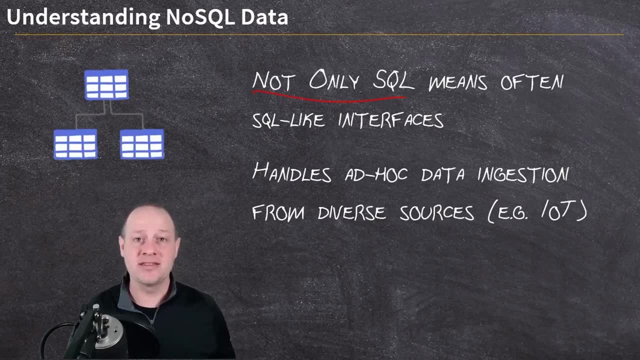 pulling in all of this data And a lot of things can happen. They might miss data values, They might report the wrong data, The data may not quite fit the standard definition of the data that you expected inside of your data schema. NoSQL databases are ready to handle that. They're ready. 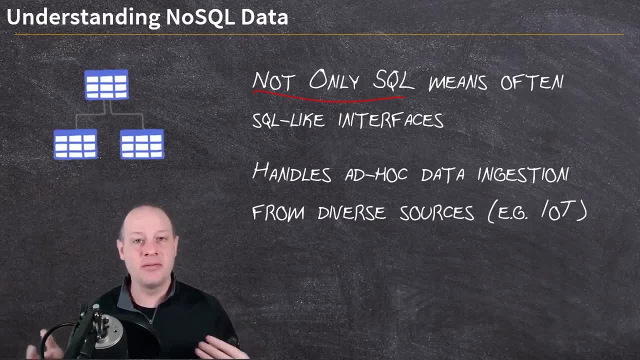 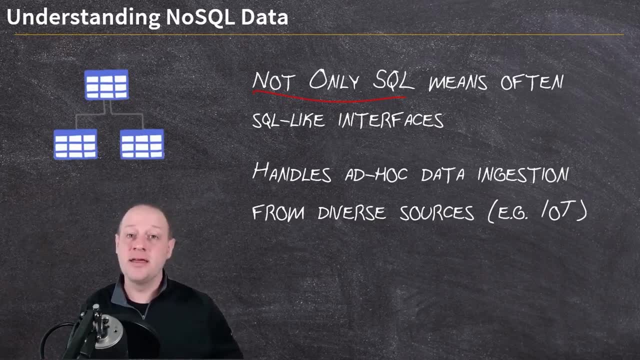 to say, okay, I can take on a lot of this different data And I'm going to be able to be flexible enough to know that, even if it doesn't fit what I'm expecting, I can still store it, capture it in some way that can be understood and read later down the line by future systems so that it can. 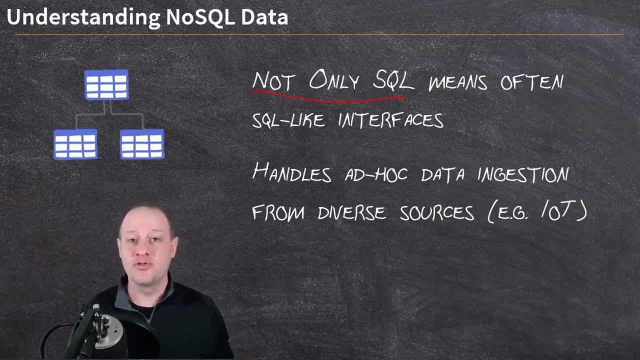 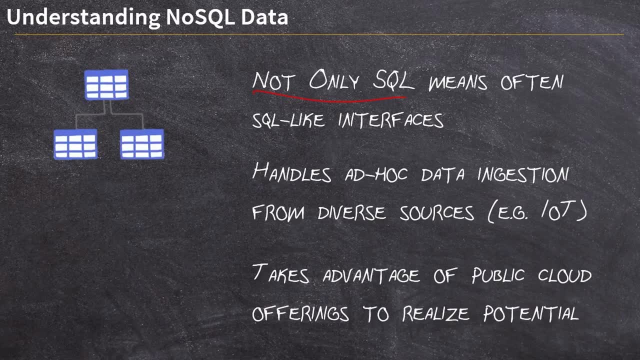 either be discarded or cleaned up or otherwise addressed in the way that it needs to be addressed. NoSQL databases also take advantage of public cloud offerings to really fully realize their potential. I think this is very, very important, because one of the things that we lose with NoSQL databases is 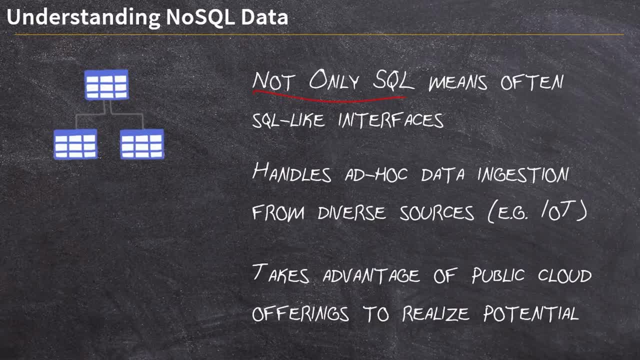 efficiency. That means we need more computing resources, more memory, more CPU power. Well, that stuff is expensive, or at least it was expensive until the rise of public cloud offerings, The ability to simply pay for what we need to use to take advantage of a big 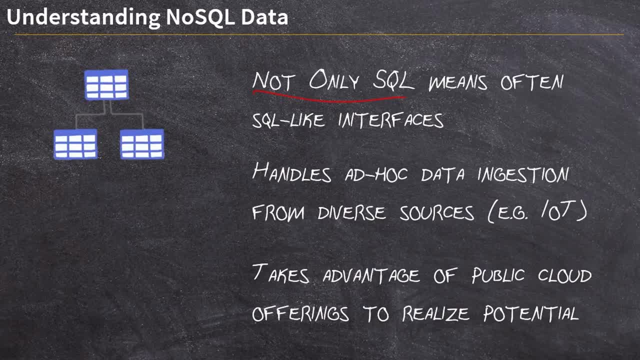 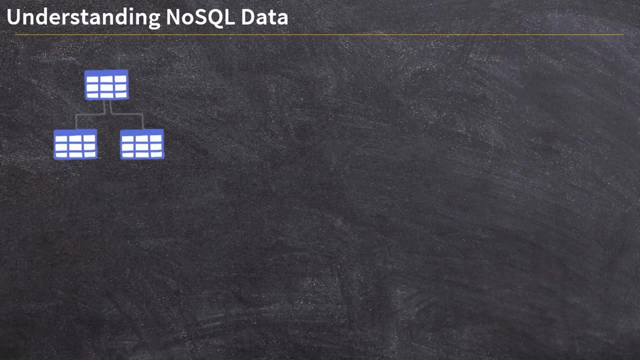 already installed managed data center like Microsoft Azure to run our NoSQL databases means that we can really get a lot of the advantages of NoSQL and minimize the impact of that loss of efficiency. Now the relational model is fairly straightforward and fairly understood. NoSQL is kind of a catch-all bucket for a lot of things that are not the 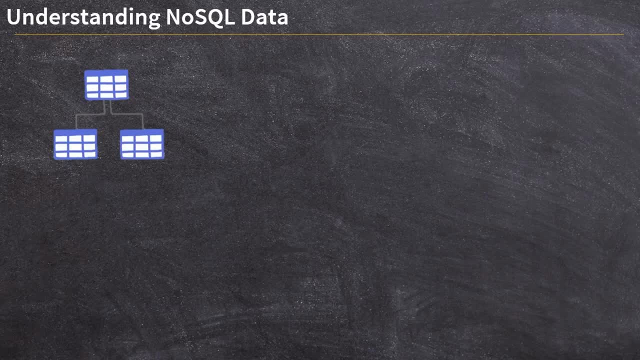 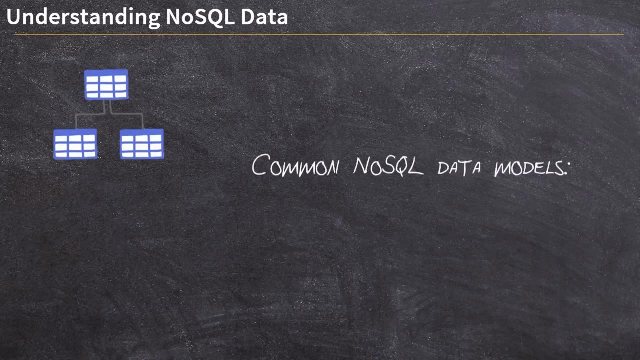 relational model. So there's well again, a million and one different ways that you might store data and call it NoSQL, But by and large we've settled into a few different standardized data models. The really popular ones that you're going to run into are going to be something called. 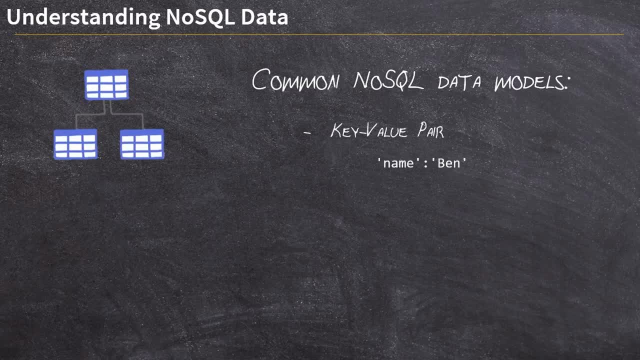 key-value-pair, NoSQL data models And they're going to be a lot of things that are going to be called key-value-pair, And this is just like it sounds like, where you have a key and a value paired up together So I can look up inside of my NoSQL database and I can say, hey, what is the? 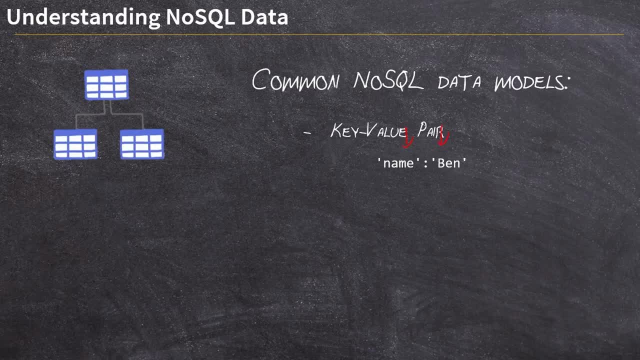 value of the name, The database will shout back to me: oh, that value is Ben. That's a key-value-pair. You see key-value-pairs a lot in memory caching. Redis cache is a key-value-pair database. You also see it in things like configuration files. right, You just have a text file with a. 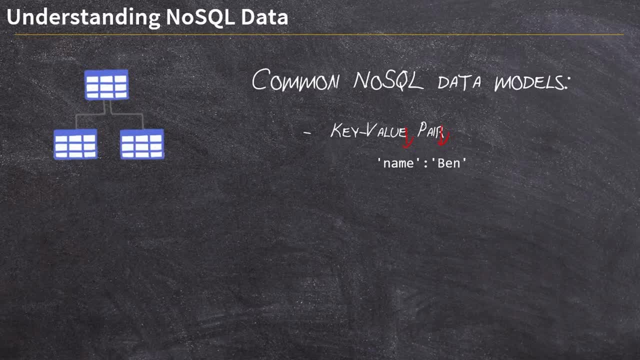 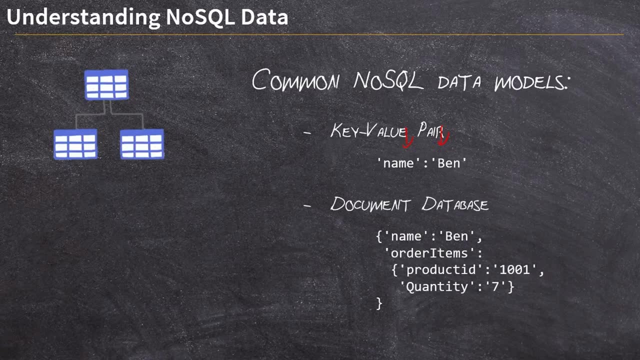 list of different configuration variables and what each of their value is. That's a key-value-pair database, The other common NoSQL data model. you run into something called a document database, And a document database is kind of like a collection of key-value-pairs that are all bundled up. So you'll see, here I've got yeah name Ben. 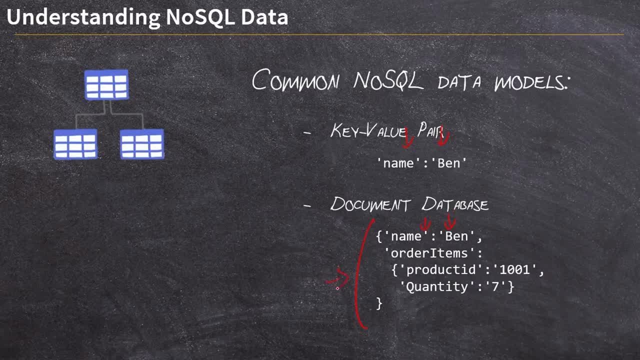 but that key-value-pair is actually part of a larger entity or a larger object that we call a document. And those key-value-pairs may not just be simple standard values. For instance, here I have a key called order items and its value is actually another document with a series. 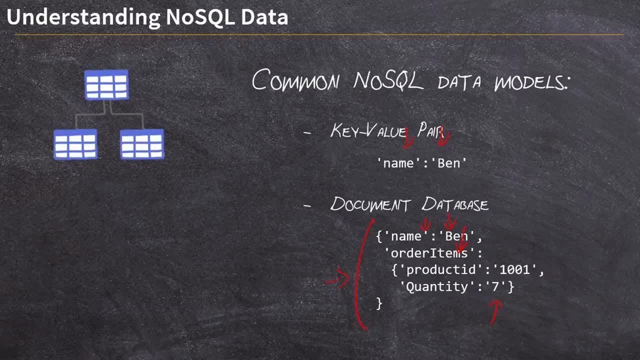 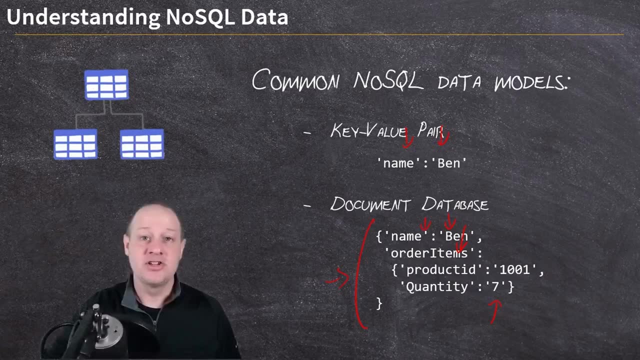 of key-value-pairs. So in a document database you may well have nested documents or nested lists, things of that nature, More complex data structures. A great example of a document database is JSON. Have you ever worked with JSON data? That's basically a document database. Another good example is an HTML. 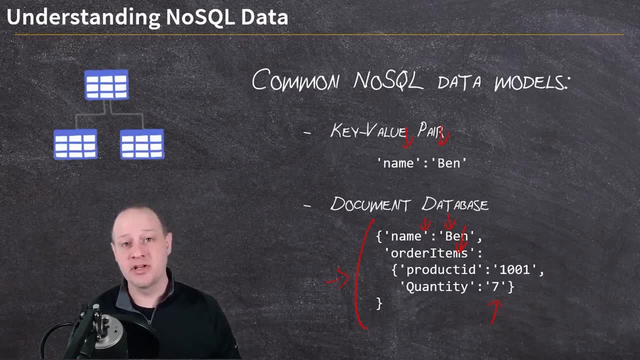 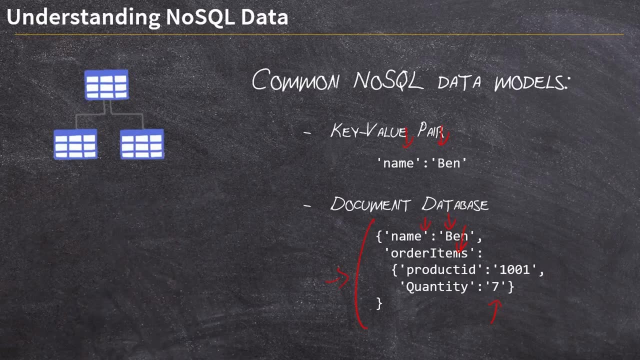 document. You may have heard of the DOM, the D-O-M That stands for document object model. That's a way to look at your HTML document and treat it like a NoSQL data document. So some other less common NoSQL data models, but still very, very important and you want. 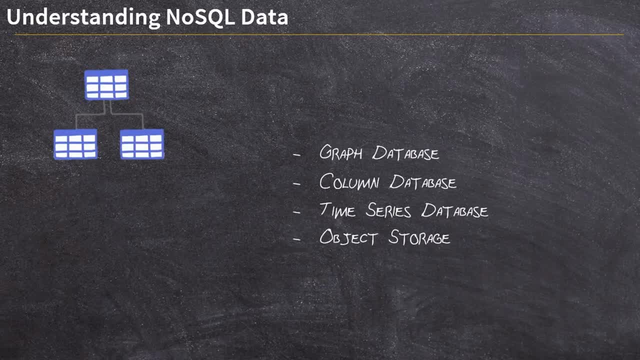 to understand them, are going to do things like a graph database, where you take those documents and you actually create relationships between them So you can understand how those different objects, how those different documents relate to one another: Column databases, time series databases, object storage, which is how you store binary blob. 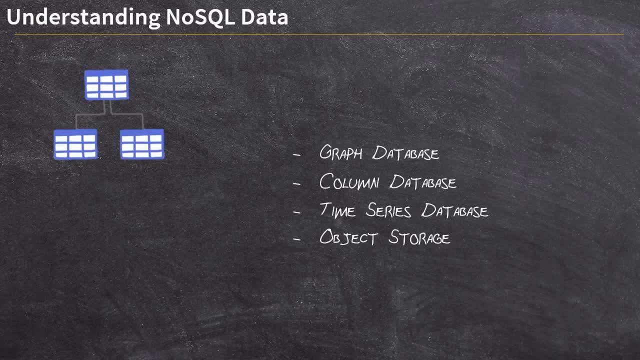 objects. Think about things like video files or media images, large binary files that don't have a lot of discrete data, but rather large, big chunks of objects that you just need to store somewhere efficiently. So all of this comes together to form the backbone of what we call. 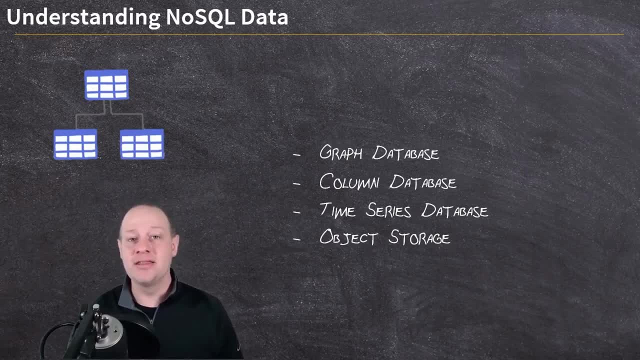 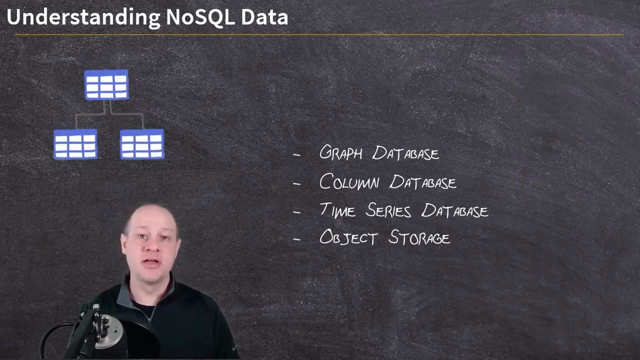 the NoSQL data model, not only SQL, And these are the ad hoc fast, less efficient but more responsive data models that are really frequently used for a lot of data operations inside of the web and inside of the cloud. these days, The most common NoSQL data model. 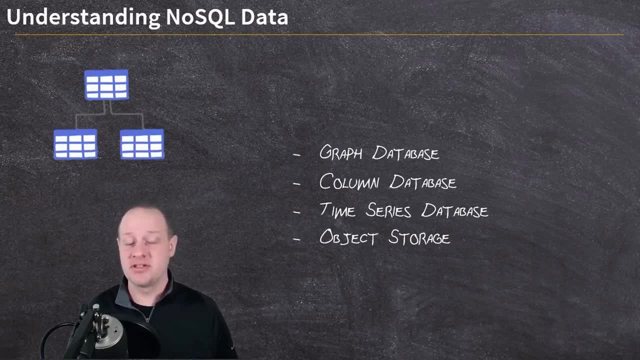 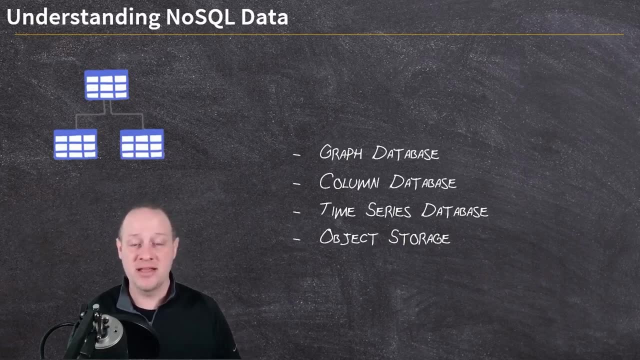 that you've interacted with is the search engine. Every time you interact with a search engine on the internet, that data is stored in the backend inside of a NoSQL structure. That is not inside of a relational database. If it were inside of a relational database, you would never be able to. 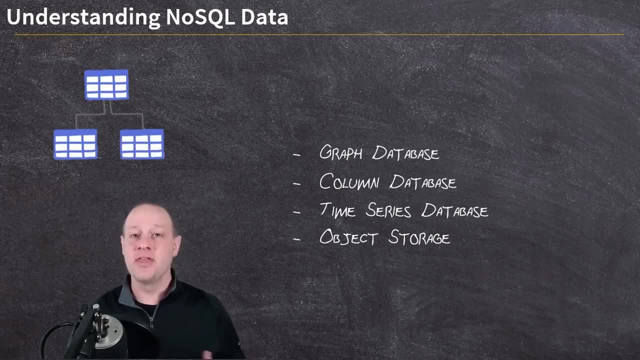 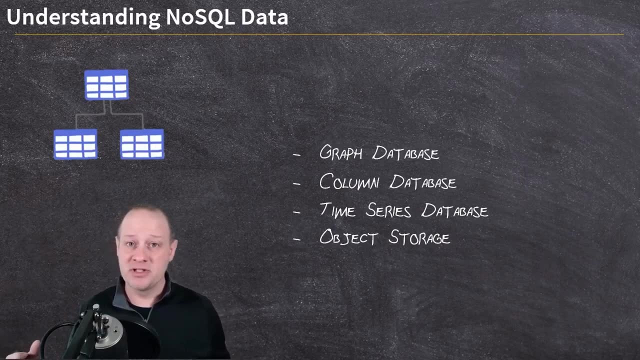 get the responsiveness. You would never get the speed out of those results that you see. So the NoSQL data model sacrifices some things. Those databases take up a lot of space. They are not especially efficient with space usage, but in return you get very fast search results, So that 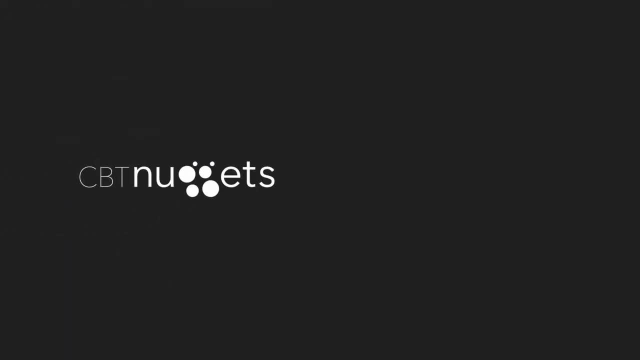 is the NoSQL data model. I hope this has been informative for you and I'd like to thank you for viewing.